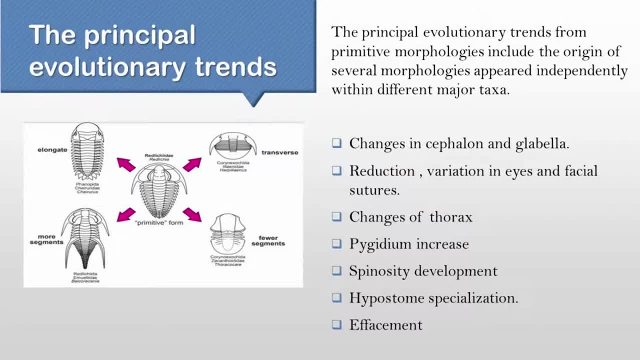 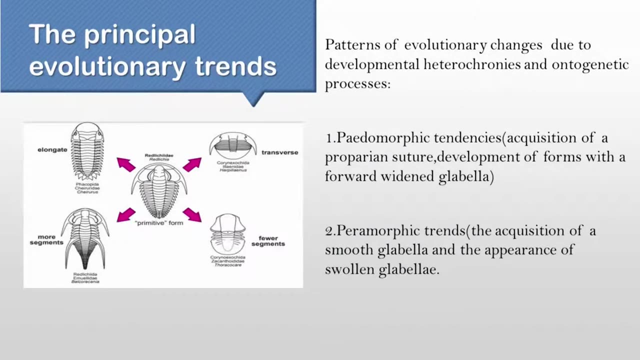 Trilobite is a sea creature that was dominant in Paleozoic era and basically an ancient arthropod. Its morphology is divided into Cephalon, Thoracic and Pigetium. Depending on their early to adult life, evolutionary trends can be divided into Padiomorphic tendencies and Paramorphic trends. 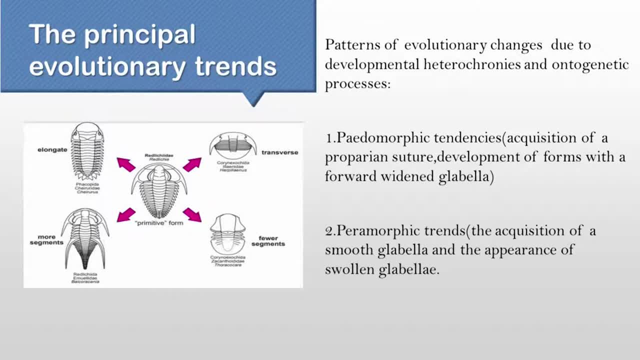 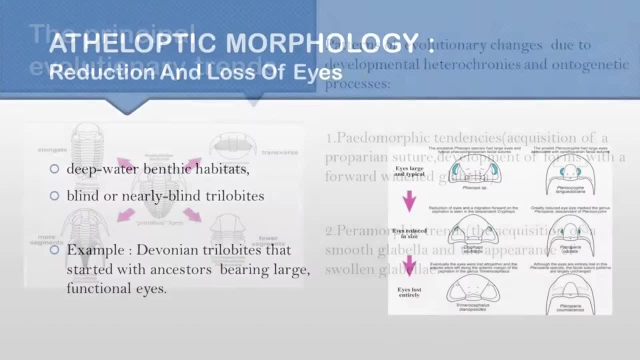 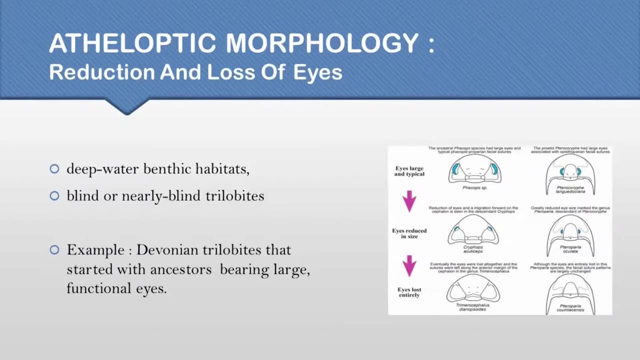 Due to change of their Cephalon eye size segment of thorax. we can differentiate them And this is how their evolutionary trend evolved. In this picture the eye size of the trilobite reduces. It was a benthic trilobite living in dim light. 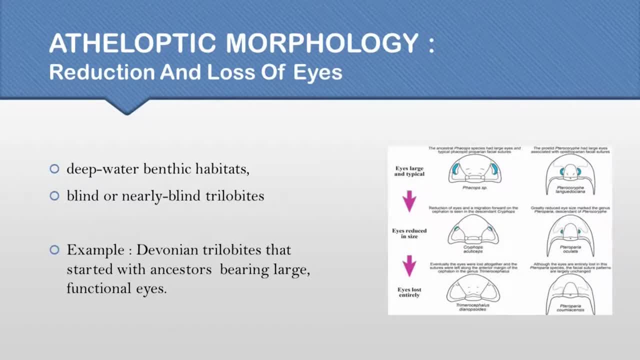 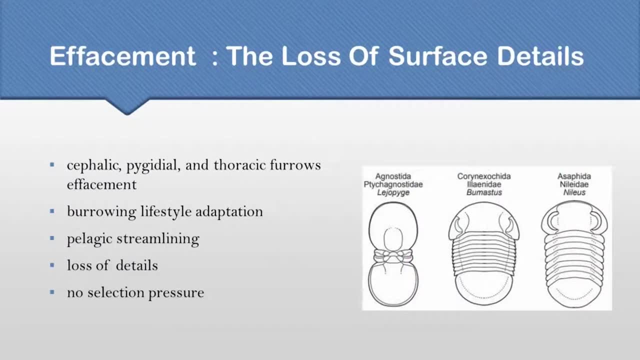 Absence of the light led them to reduced eye size and turning them blind to nearly blind. In some trilobite surface details got smoother, Like Cephalon. Pigetial and Thoracic furrows got smoothen out. 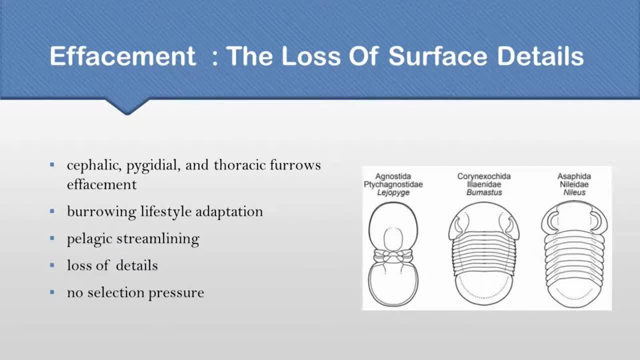 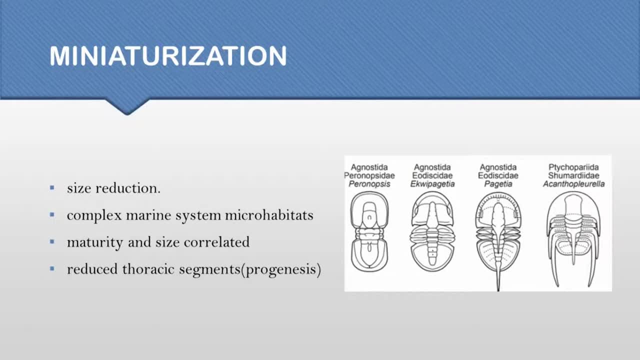 In some trilobite surface details got smoother, Like Cephalon, Pigetial and Thoracic furrows got smoother. That caused some problems in identification of some species. trilobite got smaller in size. if progenesis is present in that trilobite. 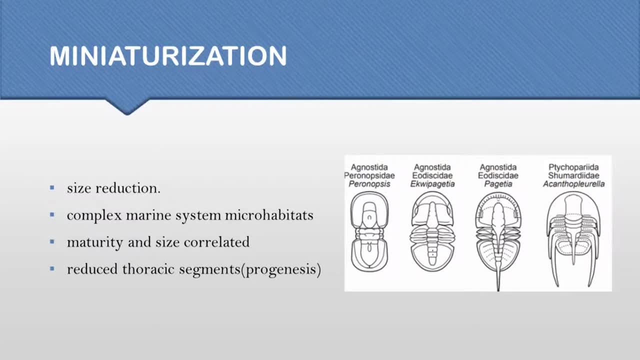 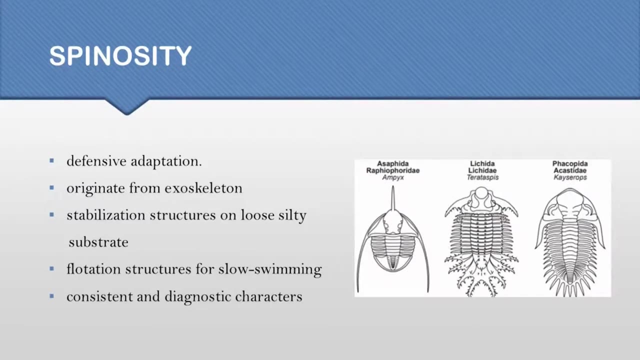 species. then miniaturization occurs in thoracic segment and also the size of the trilobite and maturity is related, like if the trilobite is matured early it will be smaller in its adulthood. spinocity is development of spines in trilobite. spines may be part of exoskeleton. their spine helps them to. 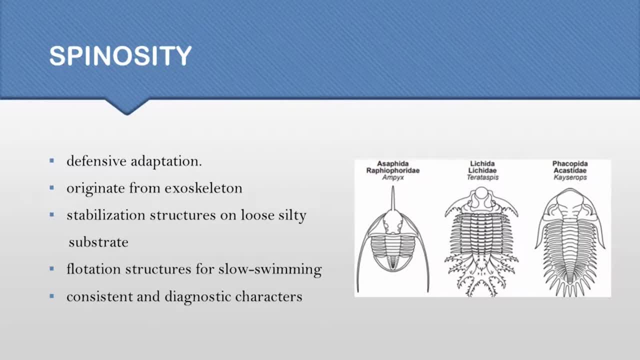 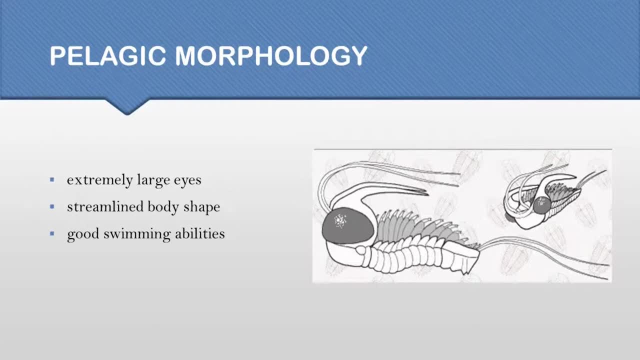 stabilize their body or to swim slowly in any environment. in case of pelagic morphology- the trilobite shown in the picture- they evolved their body to survive in the sea. they evolved according to their swimming strength. this evolution led to elongation of their body and eyes.